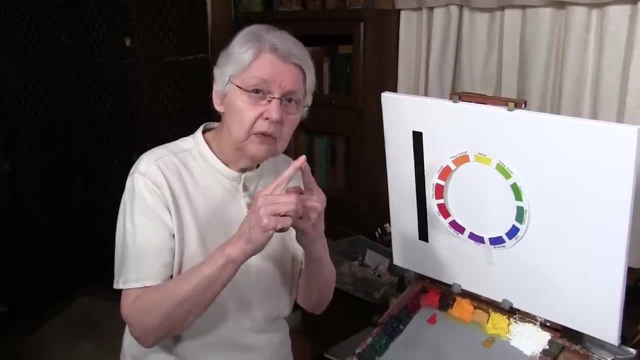 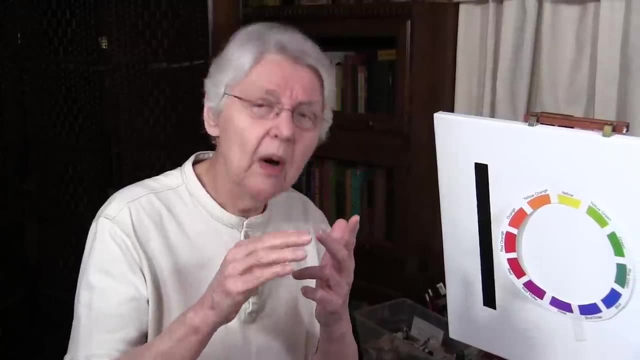 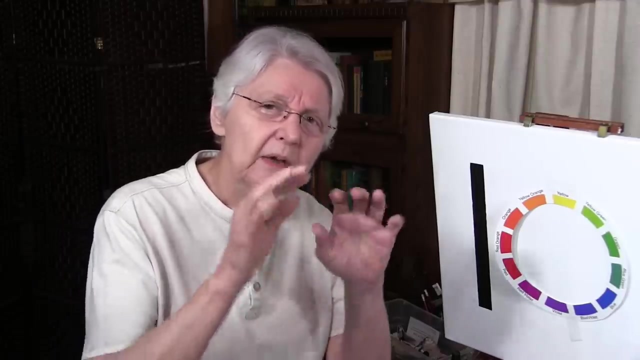 So what happens is the value of a color will change, The intensity and chroma of a color will change, Or the hue of a color will change, And sometimes all three of those things can happen at once. Let's forget hue and intensity and let's just focus on value. 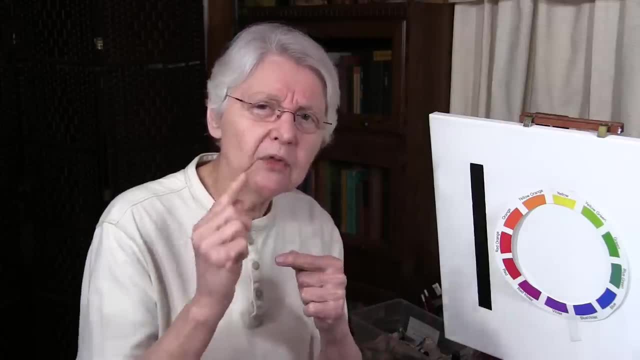 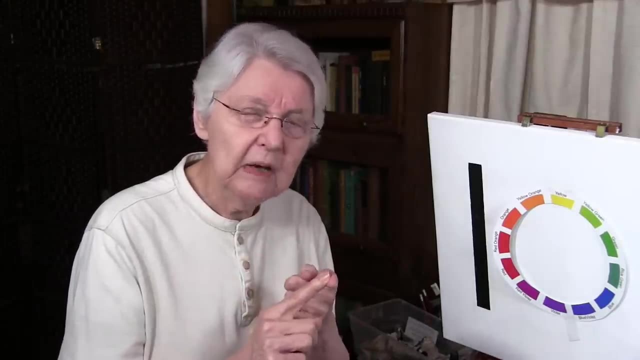 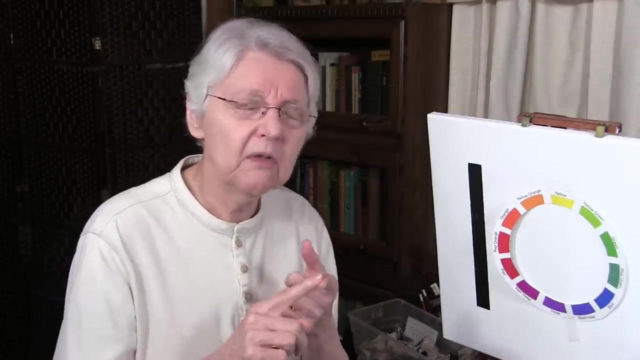 Now, how can we focus on value without focusing on intensity? The viewer said: use the word intense when he said that a dark red seems more intense than a dark yellow. Yes, a dark red seems more intense than a dark yellow. I believe that's what he said. 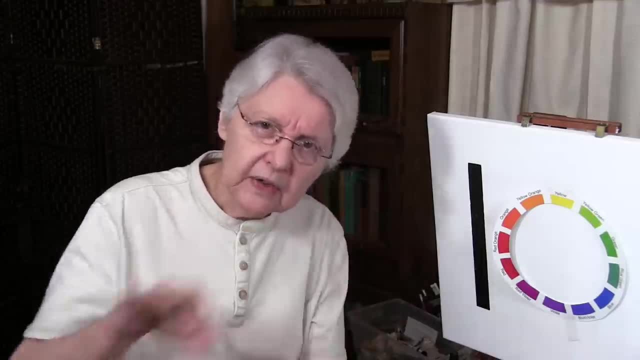 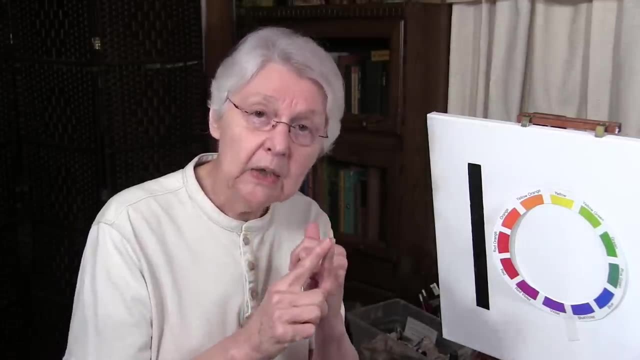 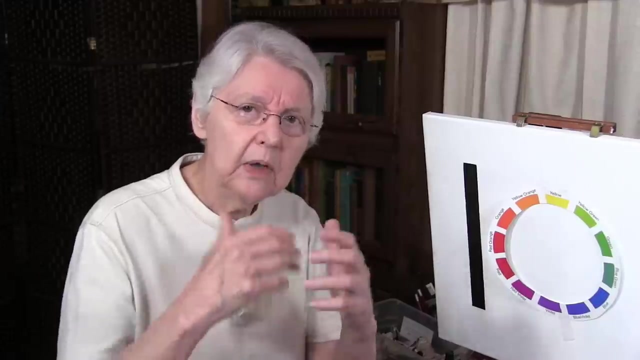 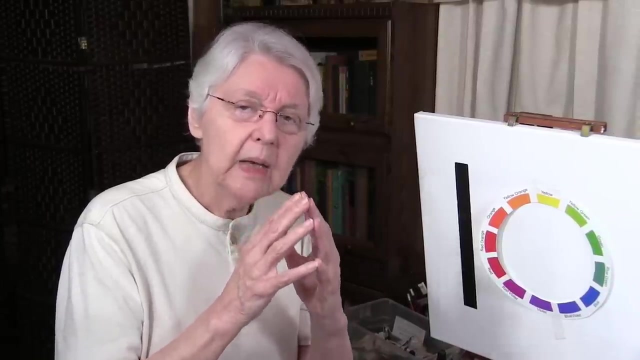 Okay, Intense is the wrong word. Let's get that word out of the way because that's more confusing. Try using just the terminology of light or lighter and dark or darker, Just those two words. So any color, when it changes- or well, you might say, in its original form- is going to start out as either light or lighter than other colors, or dark or darker than other colors. 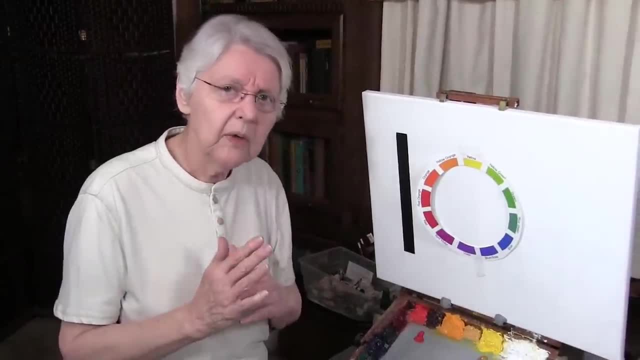 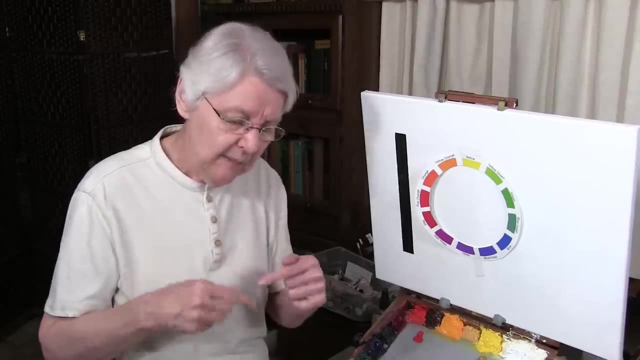 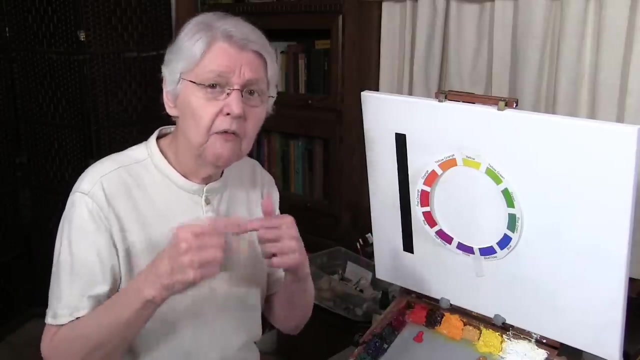 Now we're accustomed to the color wheel as our guide for working with colors, So let's just start with the color wheel Now. the color wheel is made of what is pretty much considered to be a consensus of the true hue of a color and the true value of a color. 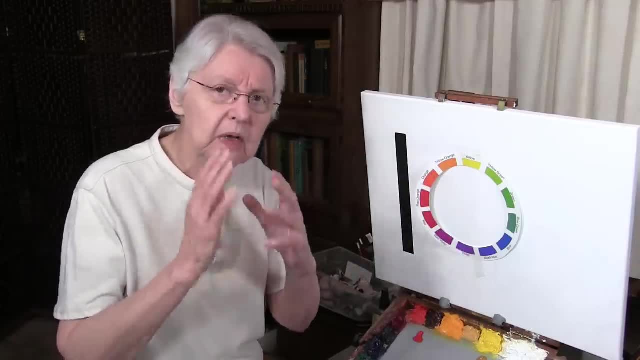 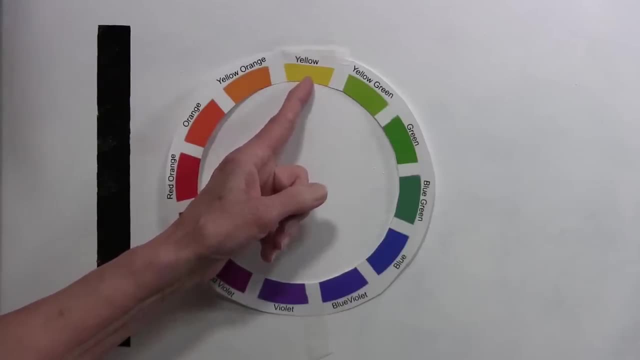 So as yellow as we would read yellow as a local color, you focus on yellow here. Is yellow lighter Or darker, Or darker than yellow green? Is yellow lighter Or darker than yellow orange? Now, if you squint, squint at the color wheel here, what do you see happening? 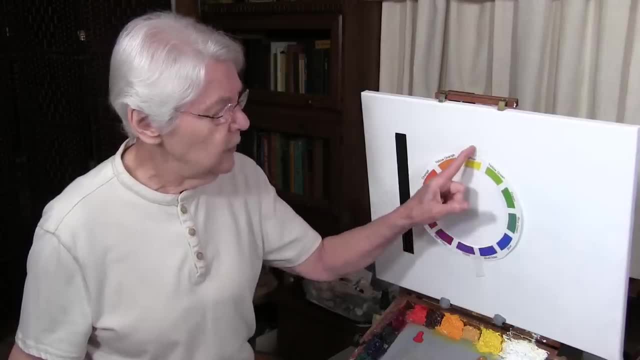 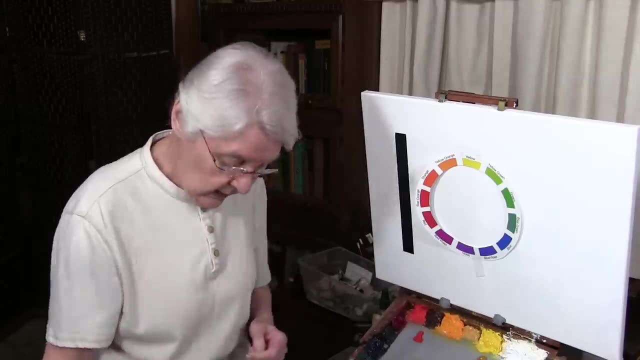 You see this yellow blending in or being more akin to the white. White is the lightest- you might say the lightest of our colors. Black is the darkest. Now let's do a little experiment here, One way that you might play around with this: 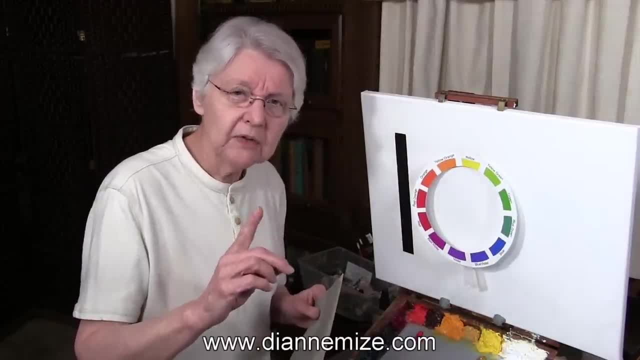 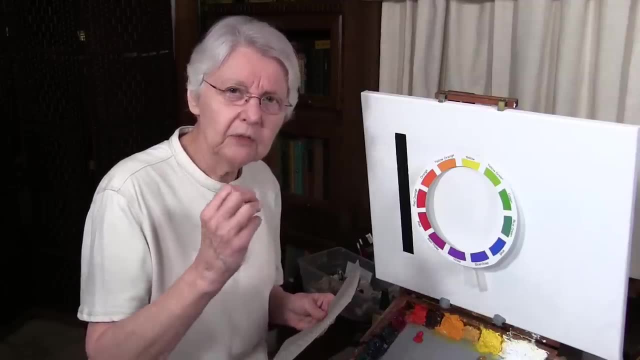 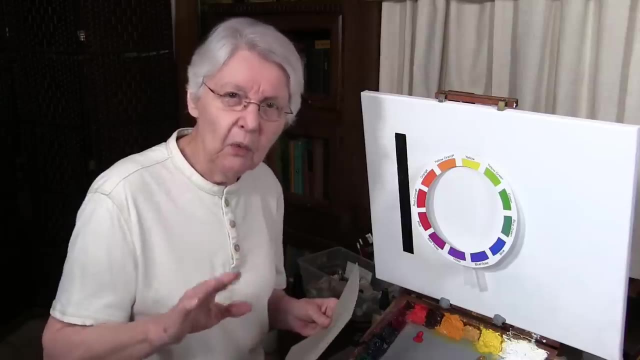 Go to our website, dynamizecom, Click on free materials And add to your cart the color wheel, the one that is balanced. It's hue, intensity and value. balanced color wheel. Order that It will be free, It won't cost you anything. 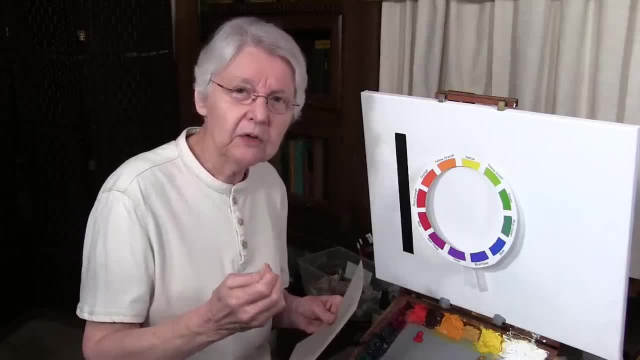 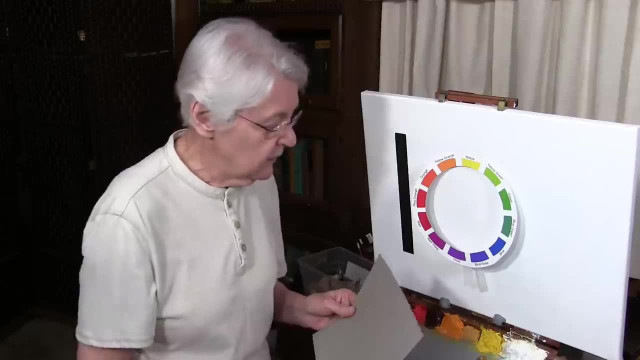 Print it out by following the printing instructions, And you then can cut out the center of that and play with some observations of color. Alright, so first of all, here's what I'm going to do. I'm going to stick a gray, or you might call this neutral. 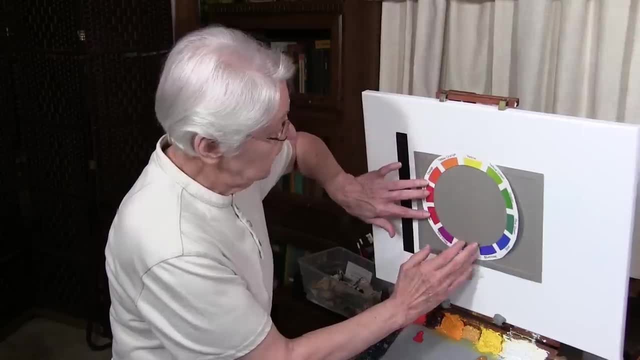 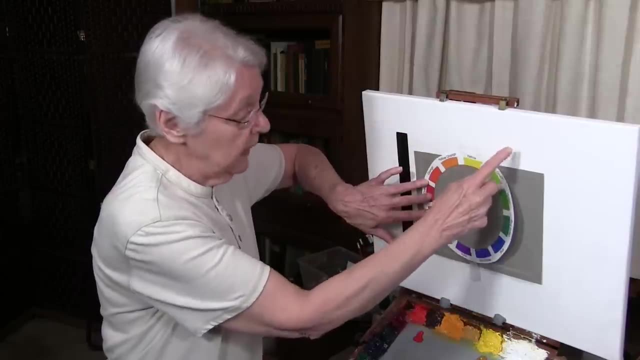 This is halfway between the blackest black or the darkest dark and the lightest light. Now, here is the darkest dark black, Here is the lightest light of the canvas, And this is sort of in between in value. Now squint at the yellow. 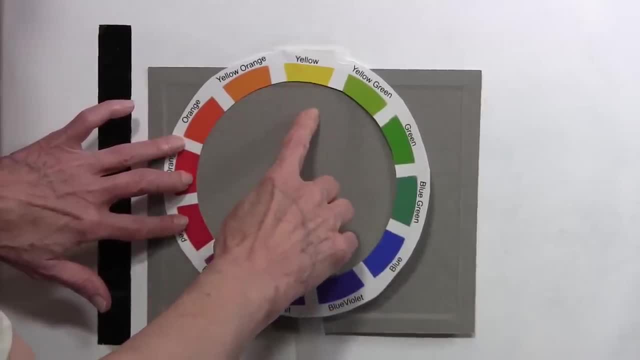 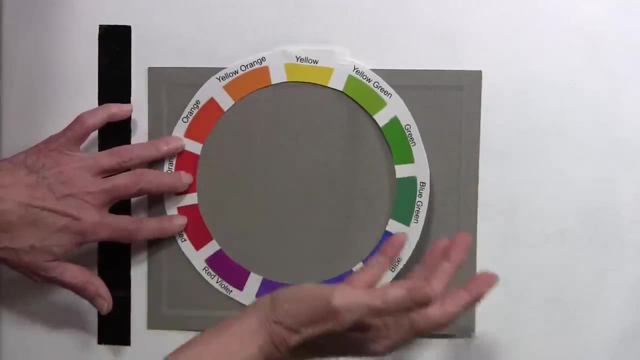 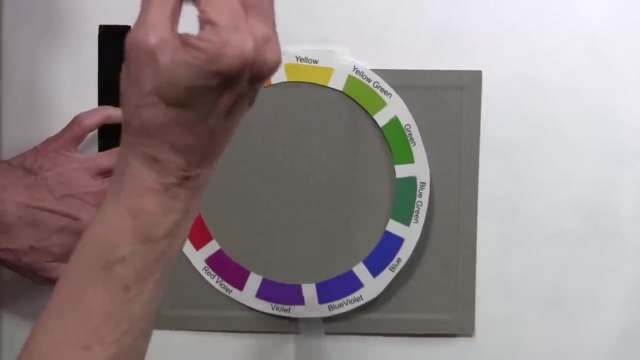 Is the yellow lighter or darker than this? Lighter Now, What about yellow orange? Is yellow orange lighter or darker than this? You squint, You see it's still a little lighter. Look at yellow green. Squint. When you squint, you can begin to. the things sort of merge together. 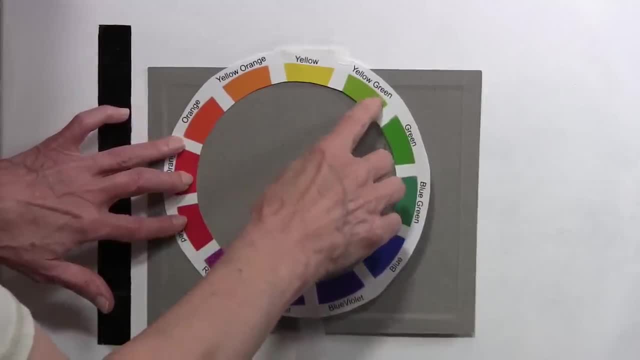 Yellow green. Is it lighter or darker? You can see it's still a little lighter, But then when you go to this green on the color wheel and you squint, you see it begins to blend a little bit more, And that way we can tell. 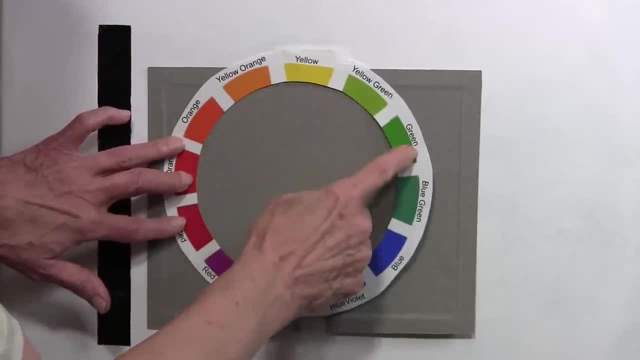 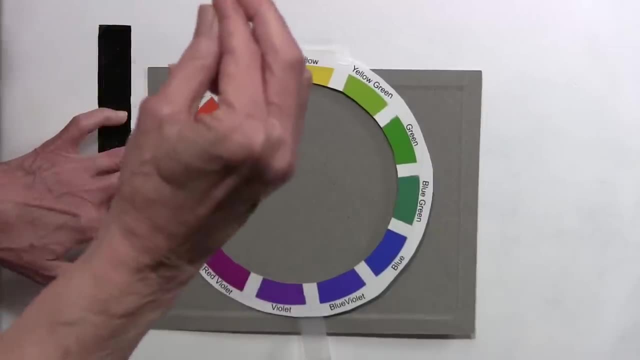 because this is much lighter, This is less light, This is less light, or you might say darker. By squinting and comparing those, we can tell a little bit more about what the inherent value is of the color And if you'll notice as the things move on the color wheel. 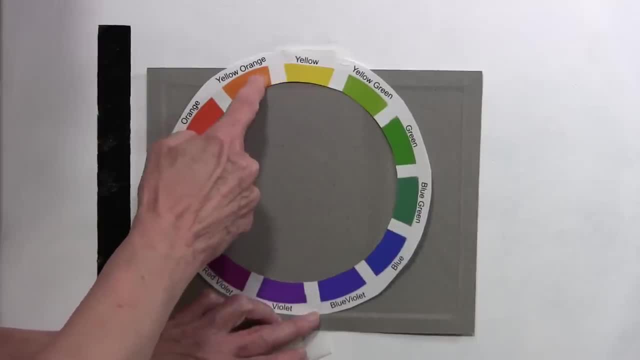 they, as colors move away from yellow, they get a little bit darker. When you squint against this gray, you can see it. They get a little darker And a little darker, And a little darker And a little darker, Till they reach about blue, violet or blue. 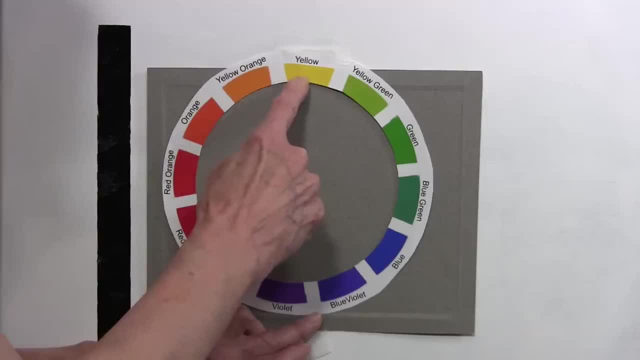 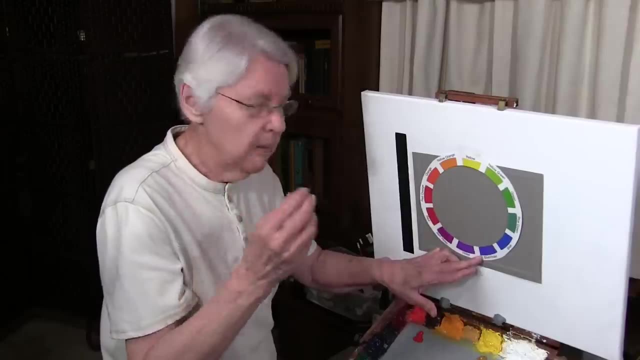 Well, you might go in this direction. You can see that the colors do the same thing. As the colors move away from the yellow, they get a little darker. So each color as it's on the color wheel does have its inherent value. 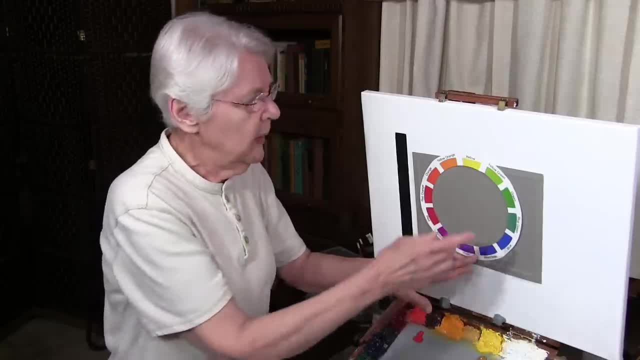 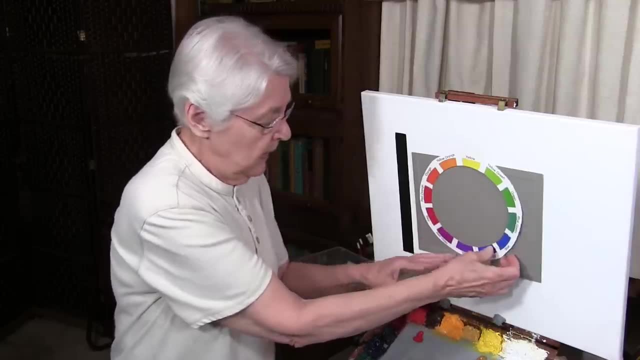 But the way you can tell that value is by comparison. Compare it to white, Compare it to gray, Compare it to black Or compare it to another color. Now let's show you something else here. I'm going to take this away. 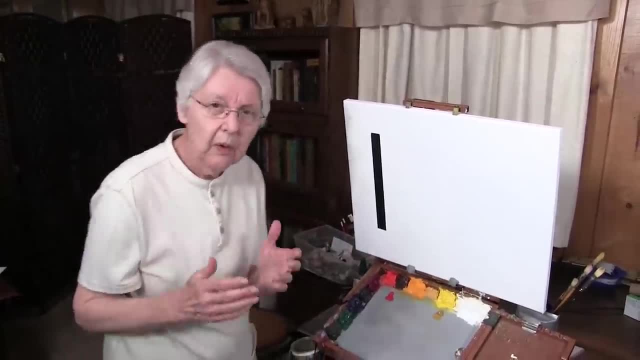 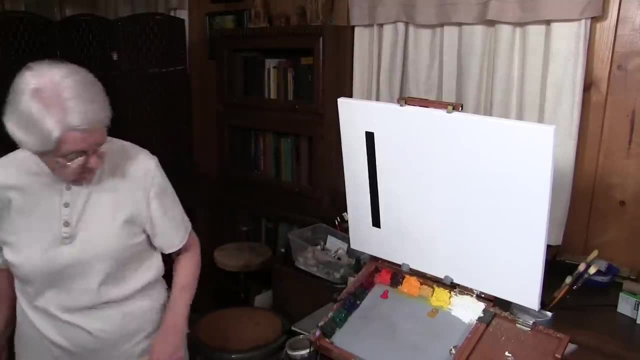 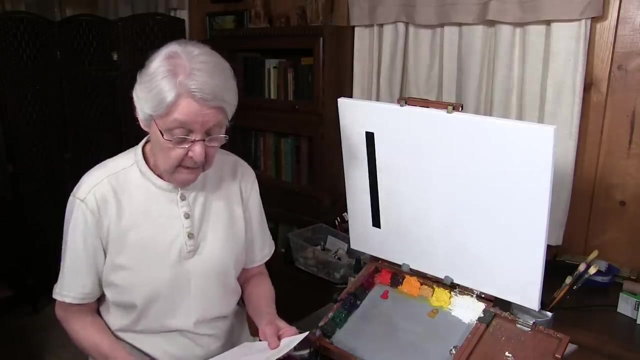 Let's look at the two colors that our viewer mentioned. The viewer mentioned a dark red and a dark yellow. Well, I think that's what he mentioned. He says a dark red seems more intense than a dark yellow. Well, let's take that word intense away. 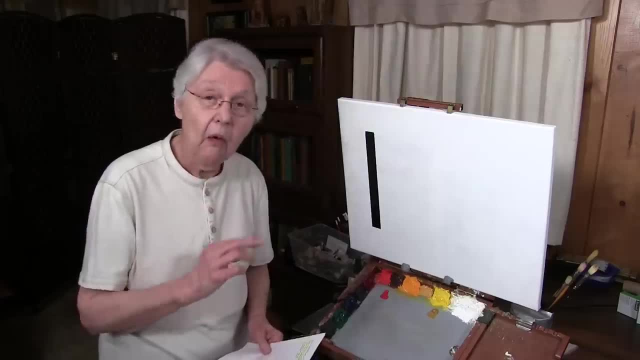 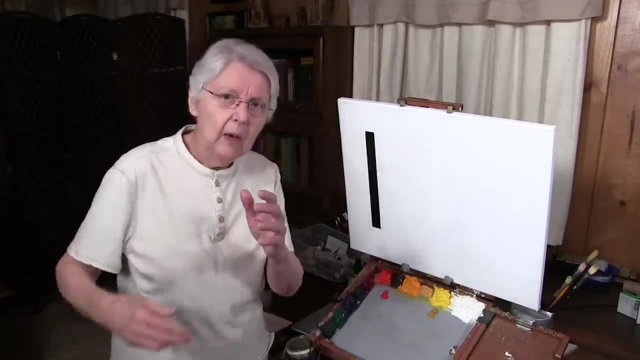 Does a dark red seem more dark Or more light than the dark yellow? The intensity is going to be another part, But if you use your method I've just shown you here of squinting- Squinting your eyes, just like this, 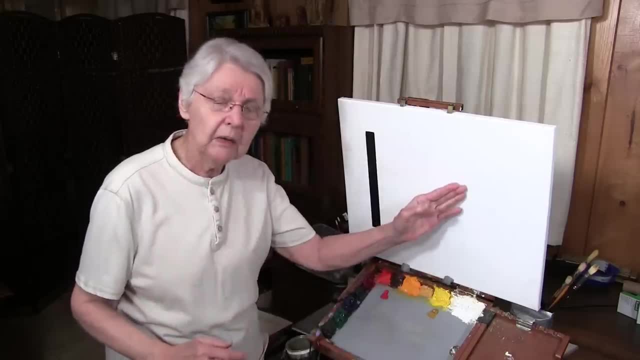 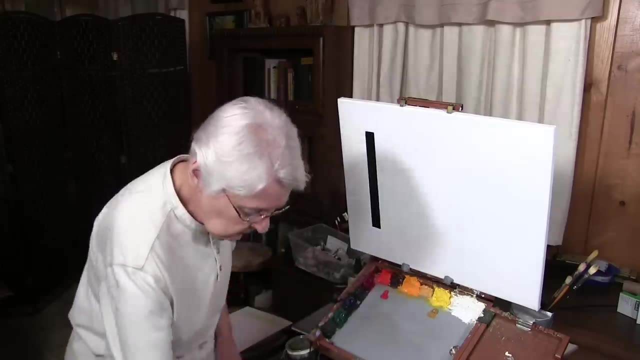 So the details go away And compare. Compare it to light, To white, Compare it to black And compare it to gray, Or compare it to other colors. You can see that Now. look on my palette. here I want to show you something. 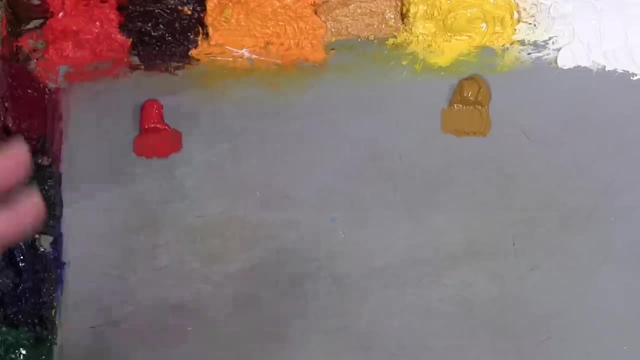 This is not really a dark red, But you might consider it a dark yellow. You might consider it darker than a really bright, really really light red If you squint your eyes. And my palette is a gray palette, A neutral palette. 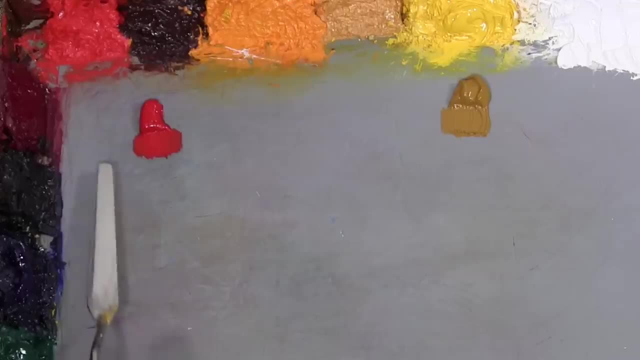 Squint your eyes and look at this red And compare it to the palette. When you squint your eyes, you see it seems to sit above the palette. Well, you go to this dark yellow. Now squint your eyes And you see that the dark yellow actually blends with the palette. 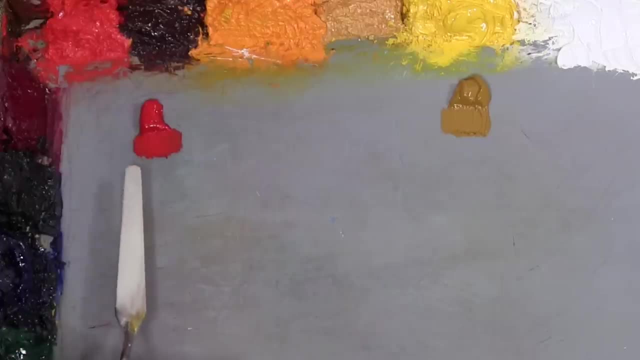 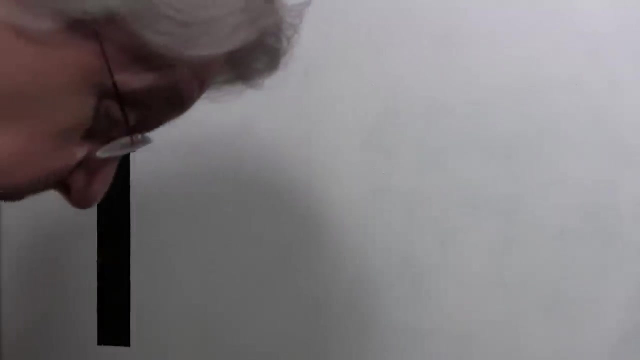 What does that tell us? It tells us that this red is a little bit lighter Because it sits above- We can see it sitting above- A little bit lighter than this yellow. Now let's compare them on the canvas. Here's the red. 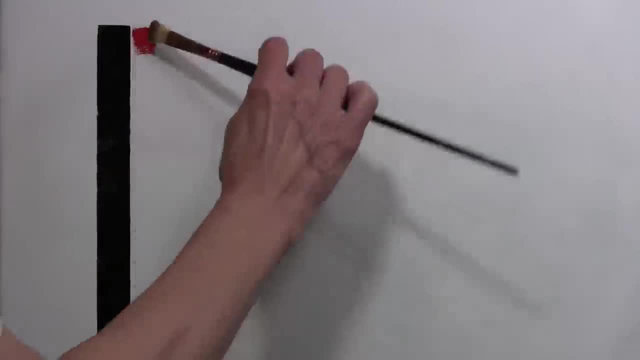 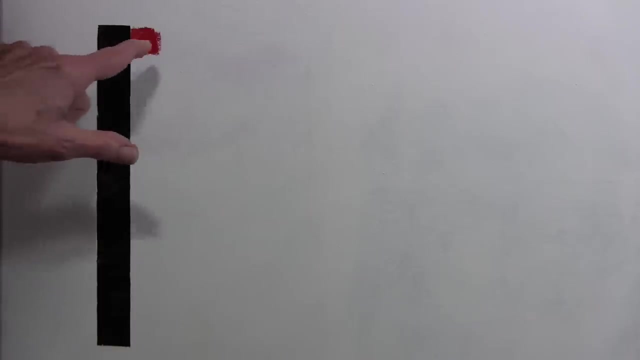 I'm going to put it right here So that we can see it compared with black. Now, if you squint, You squint And you can see black is darker, The red is lighter than the black, But when you compare it with the canvas, 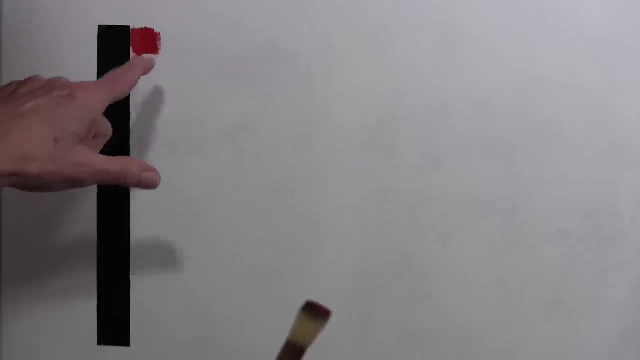 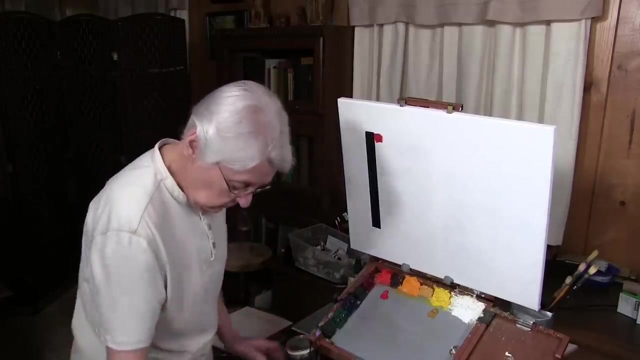 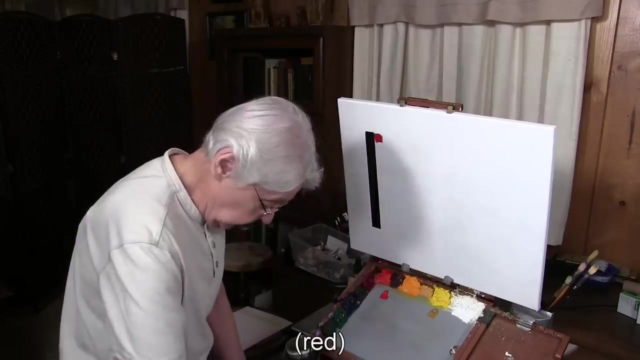 You squint, You can see the red is darker than the canvas. Now let's put the darker yellow beside it And make another comparison. Remember we're simply talking about lighter or darker, Lighter or darker. So let's get all that yellow out of the brush here. 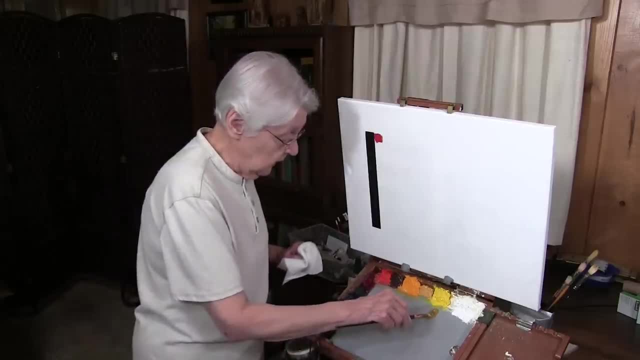 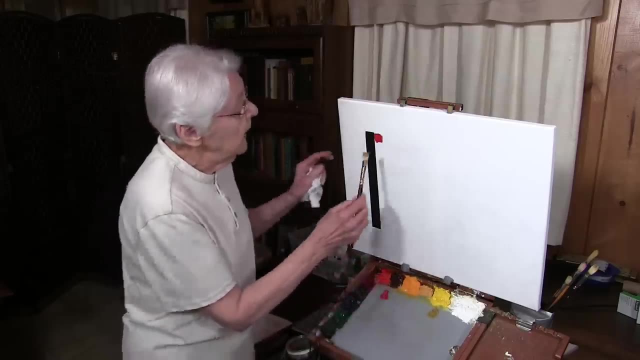 Now I'm going We'll get a little scoop of the yellow here. This is yellow ochre, by the way. It's just the traditional yellow ochre. I think it might be a Winsor Newton yellow ochre. Now, if we put the yellow, 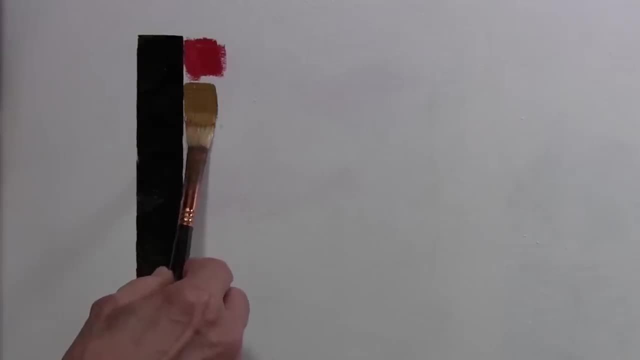 The yellow ochre, Which is a dark yellow, Put it right beside the black, Scoot it up right beside the red, Just see if I can work it there without getting too much of a blend. But I want you to see the two side by side. 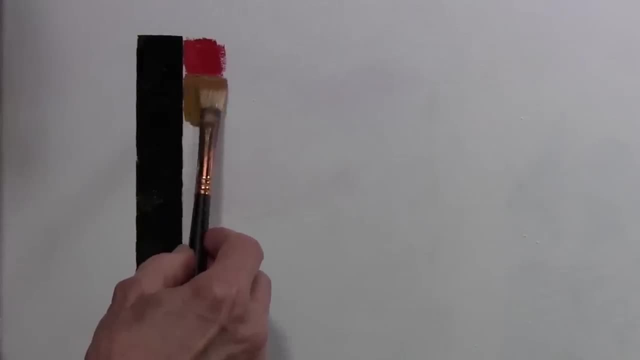 Absolutely side by side. Now what happens? If you squint And you look at these two together, You see they're very, very close in value. When you compare the yellow to the black, It is lighter than black. When you compare the yellow to canvas: 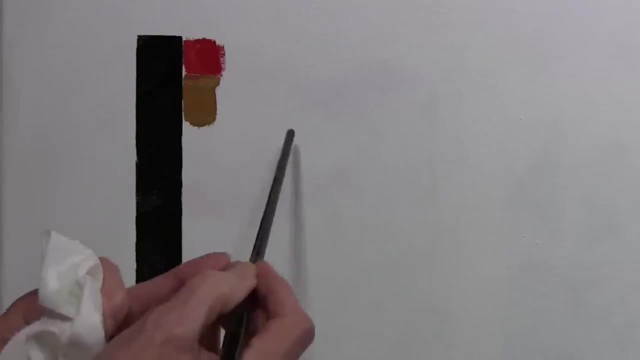 White of the canvas. It's darker than When you compare the red. It's lighter than black, Darker than white, But when you compare it to this, They're very, very close in value. Now let's do just a little bit of adjustment here. 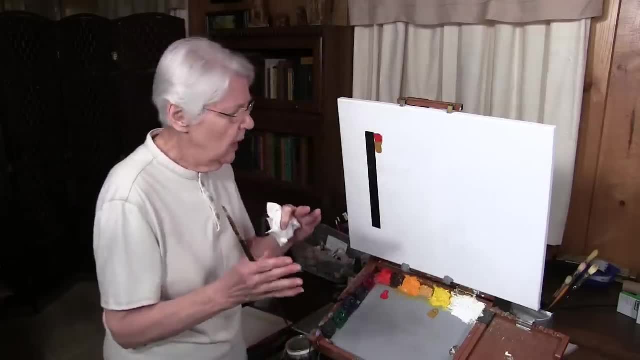 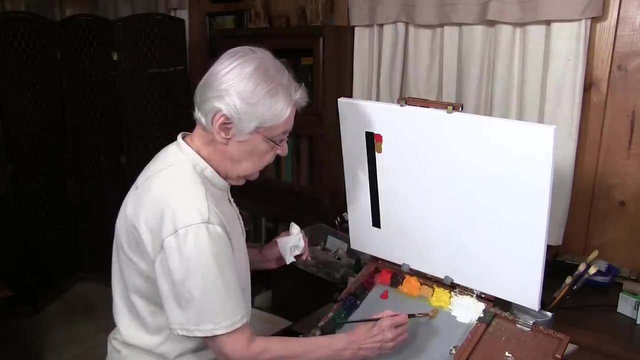 A little playing around, A little adjustment. just to show you A little bit more about how these colors vary, I'm going to take a little bit of white And add to the yellow Just a little bit. Now what happens when I do that? 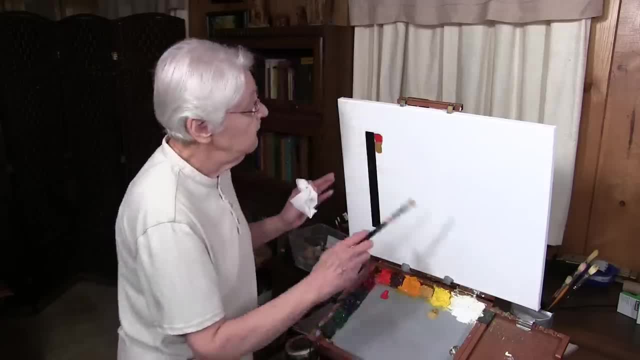 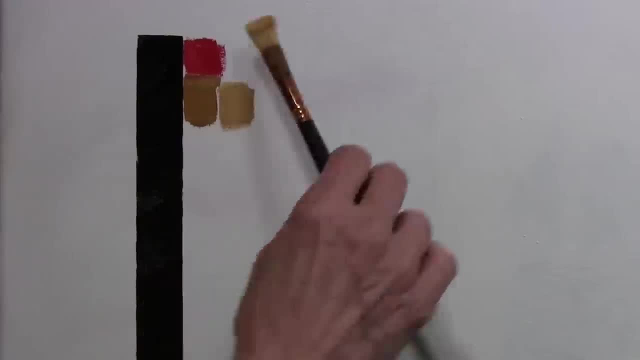 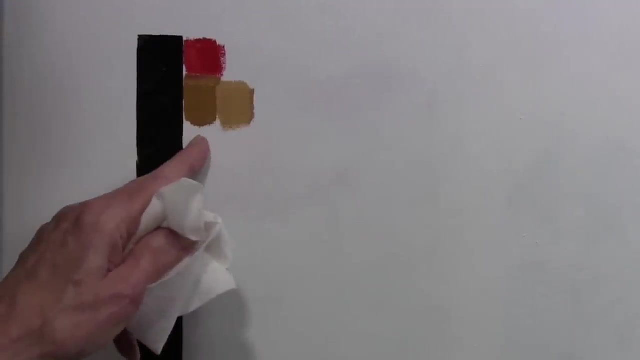 I add just a little bit of white to the yellow. Put it right beside The yellow. It doesn't change the intensity, It changes the value. Now We can see this is lighter than this, But it's darker than this. Now what if we do the same thing? 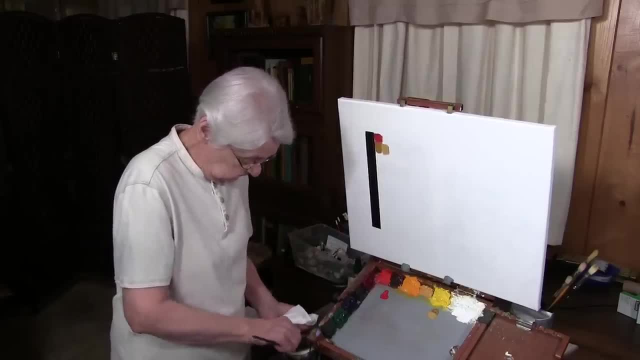 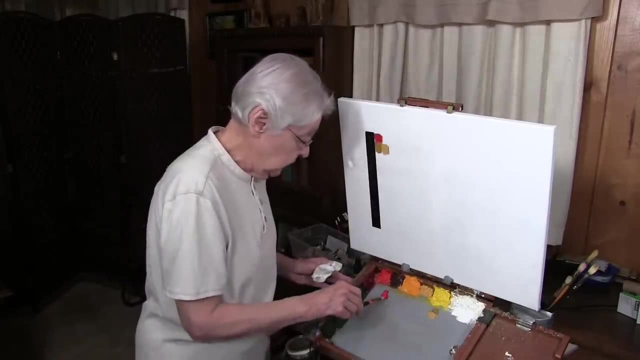 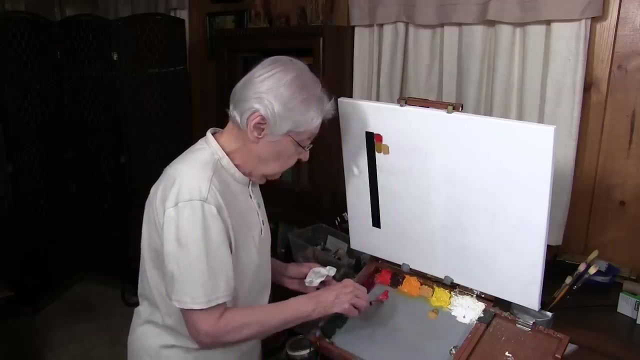 Let's do a similar thing, But with the red. So I'm going to take just a little bit of white And add to the red. We're going to need a little bit more of that. A little bit of white And add to the red. 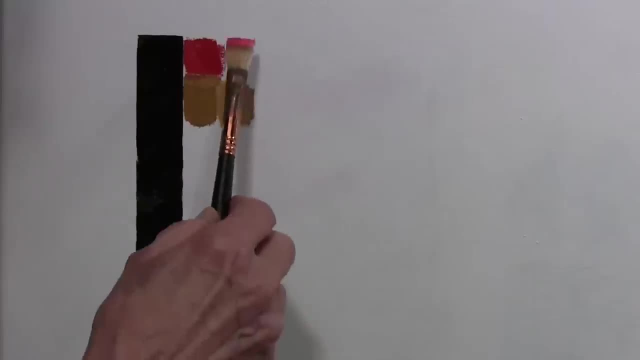 Now what I want to do here. Well, let's just see, We put it right here, Right beside, Right beside the tube. Now squint. Now, when you squint, You can see this is lighter than this, But darker than this. 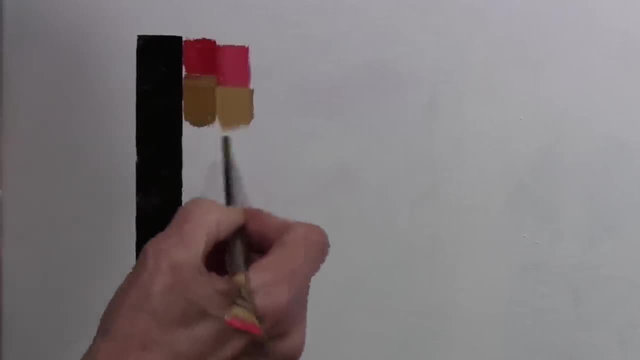 It's lighter. No, let's look at just these two. Now. when you squint with these two, What happens? You can see that this is a bit darker than this, Because this is, Feels or leans a little bit more towards the dark here. 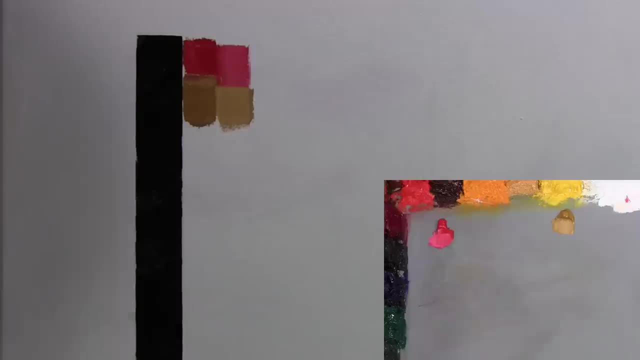 Whereas this leans a little bit more towards the light there. If we continue to add a little bit more light To that red, Let's see, Let's put it right here: A little bit more light to that red, We can eventually get them the same value. 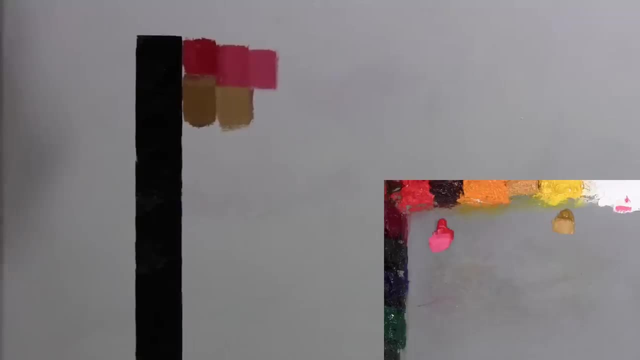 I'll go back and pick up that same bit of the Of the yellow ochre again. Now, why am I going through all this? Because these are the kinds of experiments that you can do When you're having trouble identifying color, When you're having trouble working with the value of color. 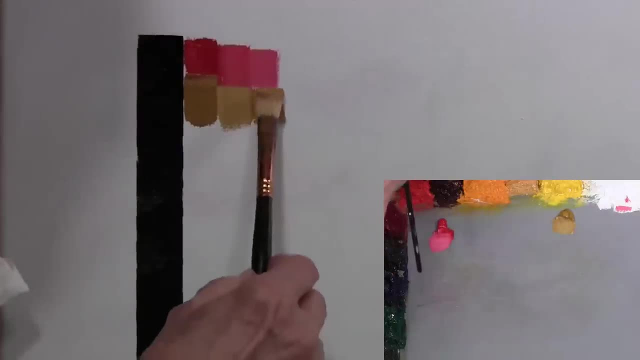 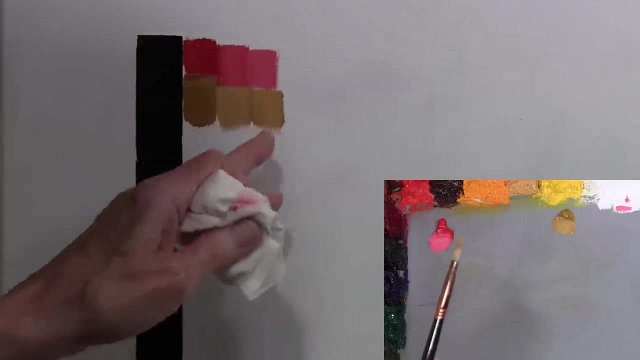 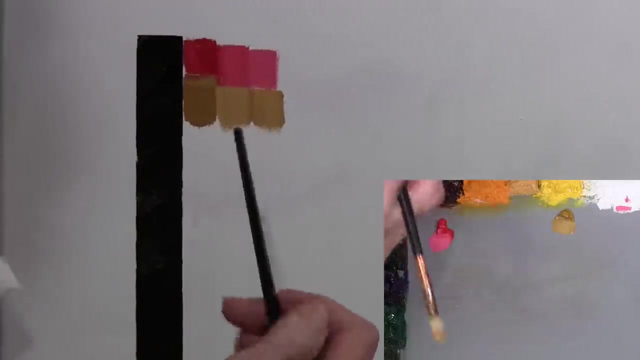 If you experiment with Comparing the values And changing the values, Okay, those two are not quite Changing the values and comparing the values Again to have that feel For the inherent value of a color. Now you can see this is even closer. 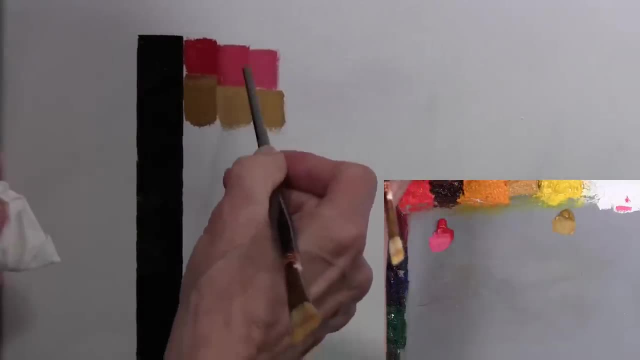 Squint, Squint, Hold the squint. If you hold the squint, See these are getting closer and closer As far as the value goes. I'm going to make one more change in the red. Before I do that, I'm going to go. 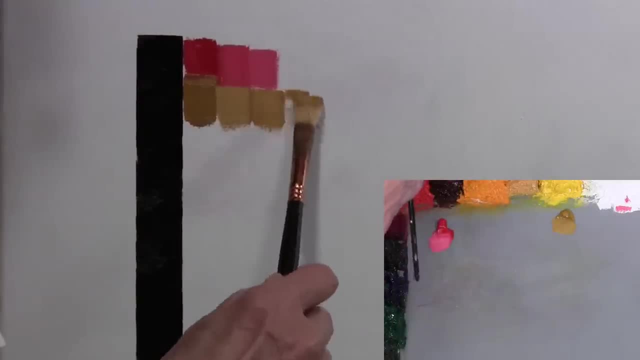 Put another little splotch of this Same value of the yellow Right here. Okay, it's the same value as this. So all of these, These three are the same value, But what I'm doing here is I'm reducing the value of this red. 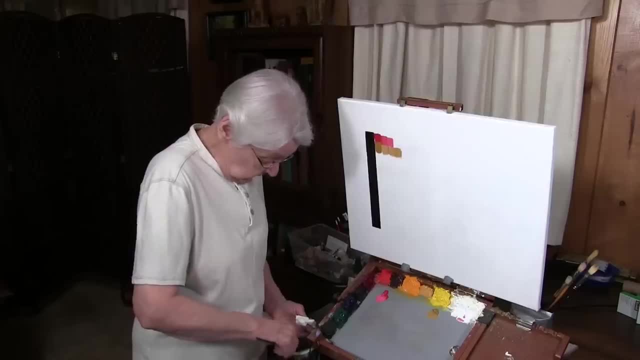 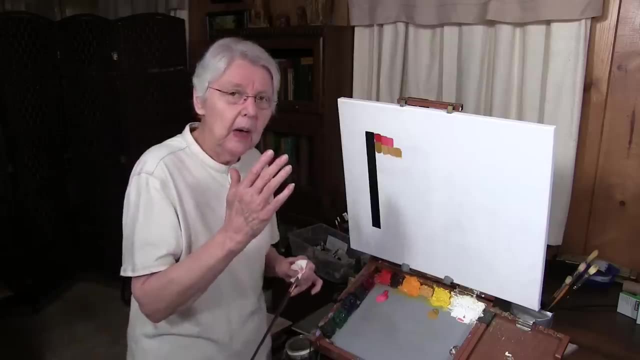 To show you that As I reduce the value, It gets closer and closer in value to the yellow, And that's how- That's one way I can tell, If Tell, the difference in the value of the red And the yellow. 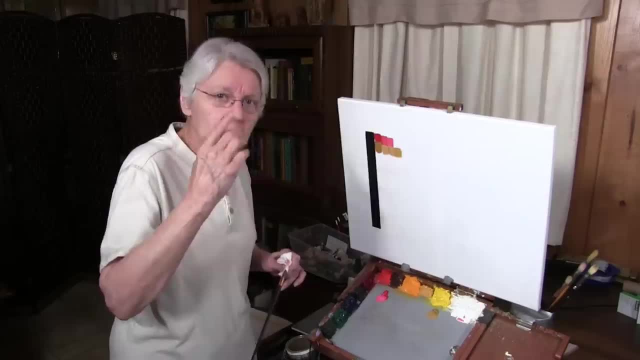 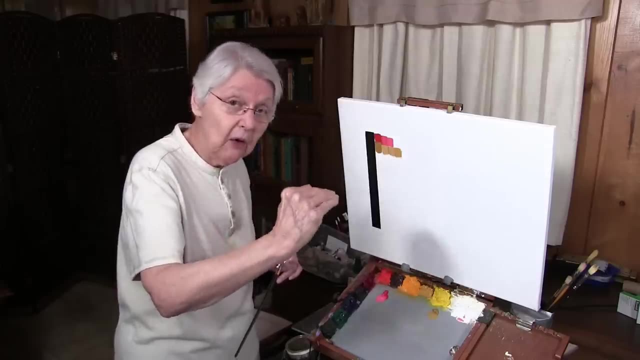 Dark red, Darker red And the darker yellow. I can just choose one, And I can reduce the value, Or I can. I can add dark to it, Or I can make it darker One step at a time, Or I can add light to it. 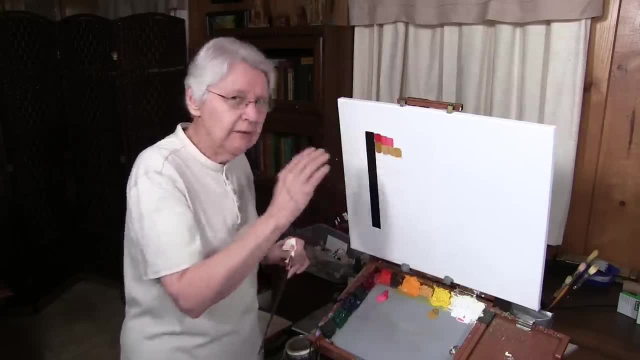 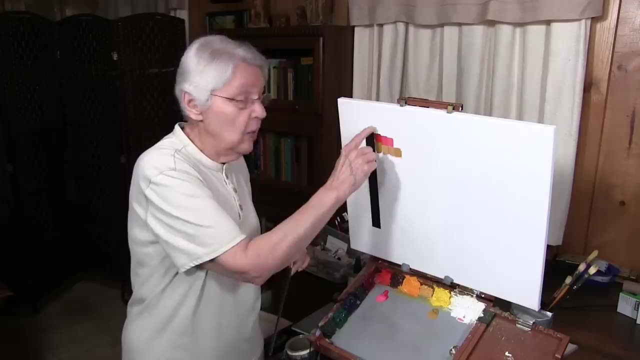 And make it lighter And then keep comparing the two. And if I'm making it darker And it begins to compare, Being the same value, Then you'll know The color was actually lighter Than this color. But if, by adding 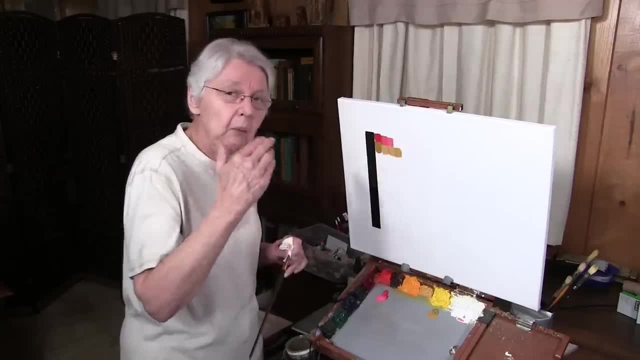 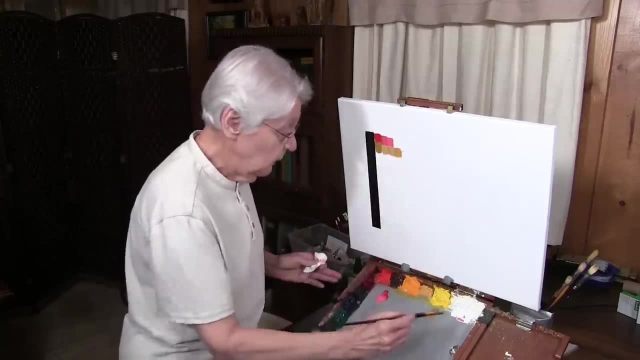 Making it lighter And comparing these two, We will know that This color is actually darker than that. So that's That's one way we can Can, That's one way that we can Study The value of color Without 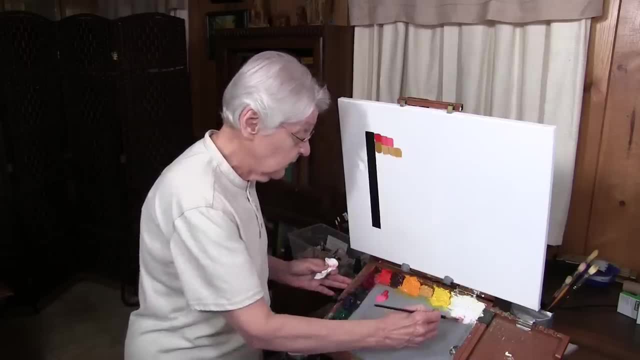 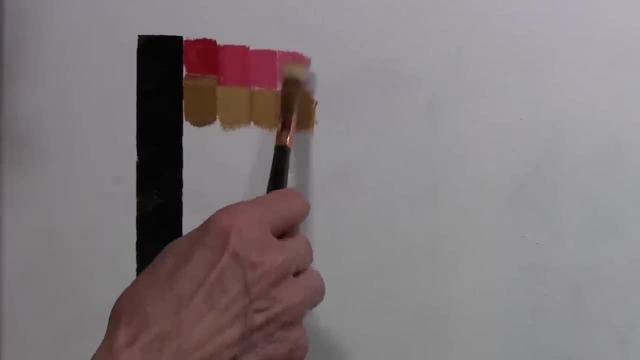 Um Well, Science, You might say, Study the value of color Scientifically. Add a little bit more light Now to that red And just place it Right here. You see, I'm just getting these By just really small degrees. 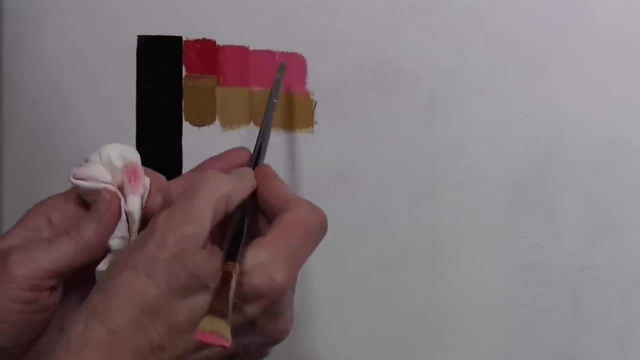 Now, If you squint, You can see These. These two Are beginning to merge Together. We don't see one value Darker than the other. As we come in this direction, We see The red When you squint. 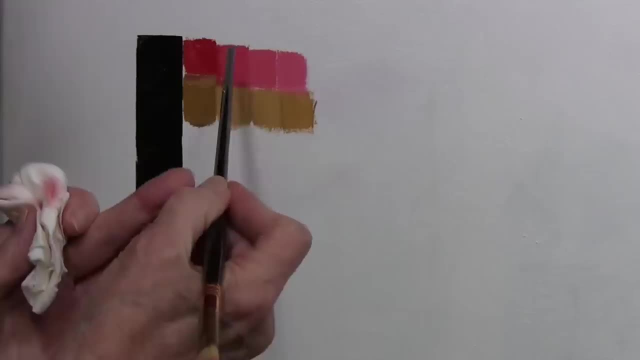 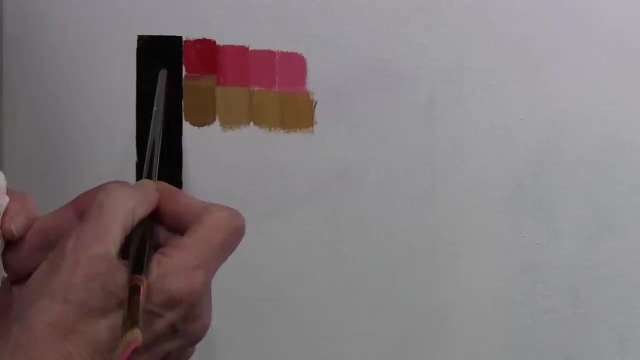 The red Sort of Jumps behind, It Is actually appearing A little bit darker Than the yellow, And so on. So, Uh, Here In their original form, We now can begin to see That the red 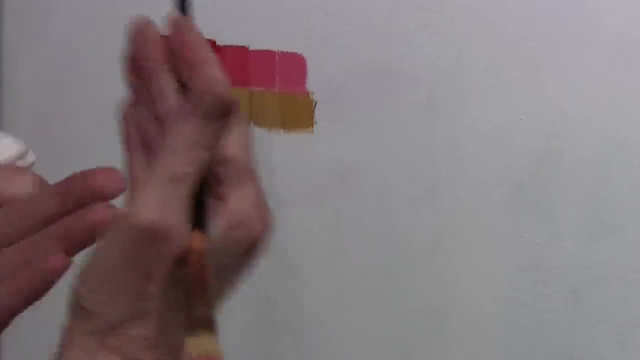 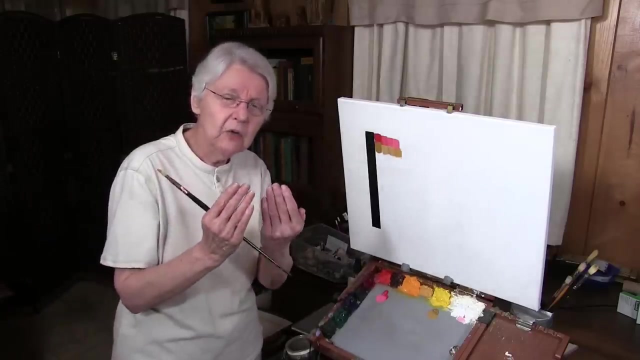 Is just a little bit darker Than the yellow Because It begins to kind of move Behind the yellow. So That's one way That you can Examine The comparison Of any two colors, If you have. Uh. 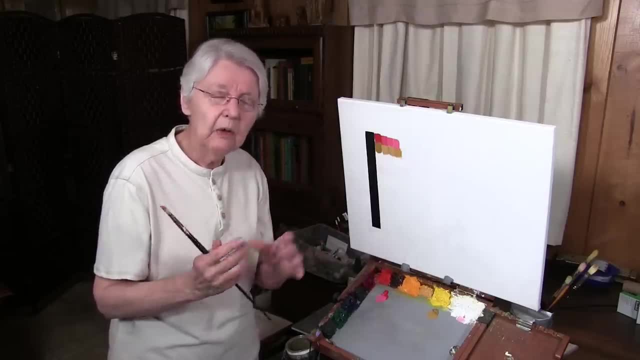 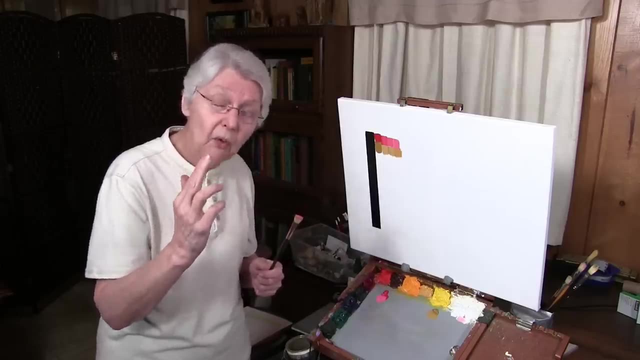 A question About the value Of the colors. Start out With the color wheel. First of all, Understand The Value Relationships Of What we might call The Colors In their pure forms, And then begin to do. 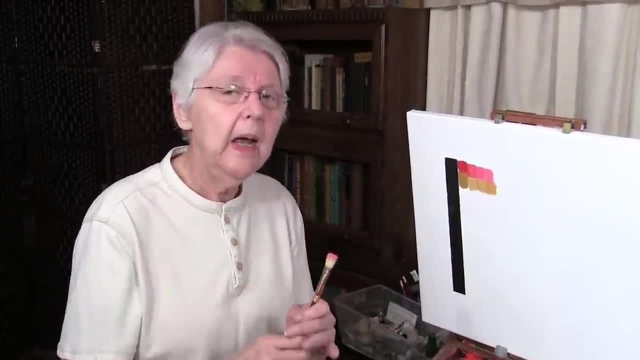 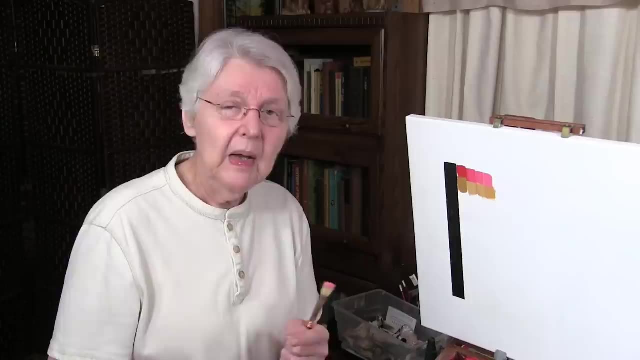 Uh, Just a little bit of a test Where you add: Uh, Choose one color, The one that seems to be darker. Add a little bit of white, One step at a time, Until Both those colors Merge Together.